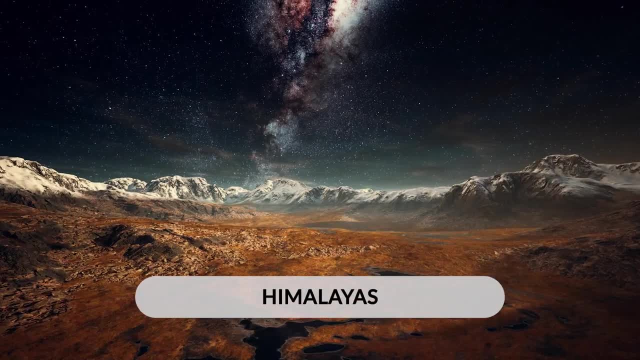 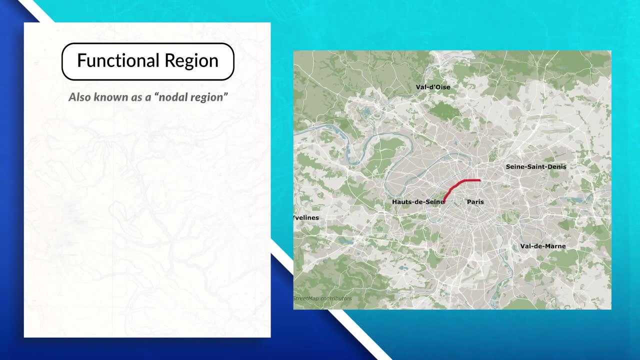 similar climate can be found across multiple countries, or the Himalayas in Asia, which are defined by a series of connected mountains. Now our next type of region is a functional region, also known as a nodal region. This is an area that is organized around a node or a center point. 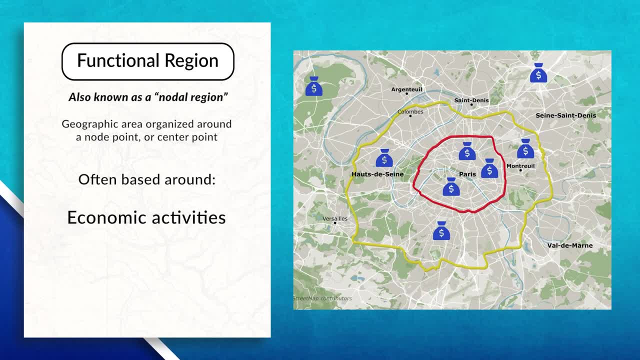 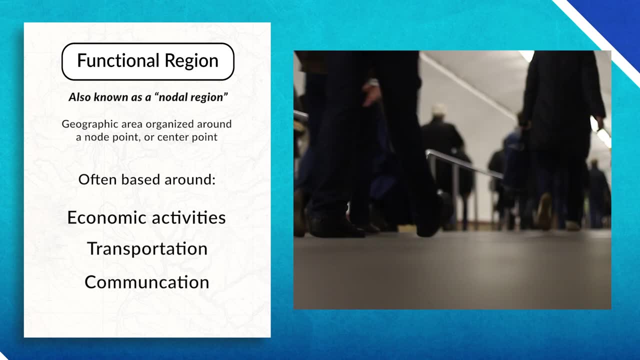 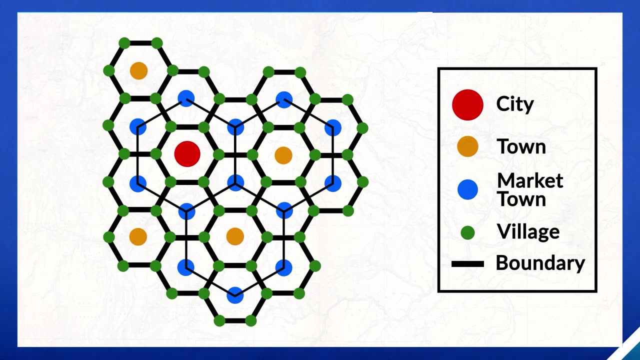 oftentimes based around specific economic activities, travel, communication. Functional regions often see the different interactions, the flow of goods, ideas or people. all tend to gravitate towards the center point of the region. For instance, we can look at the urban hierarchy of an area where a large city is often located in the center. 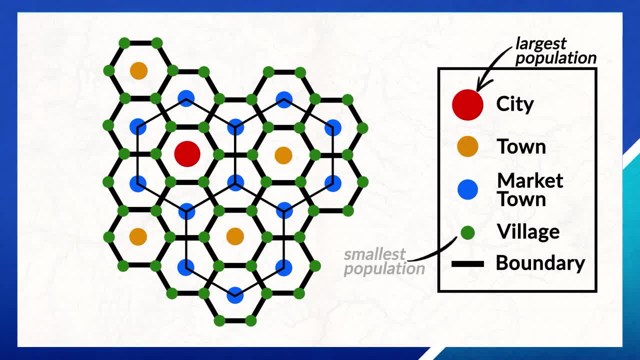 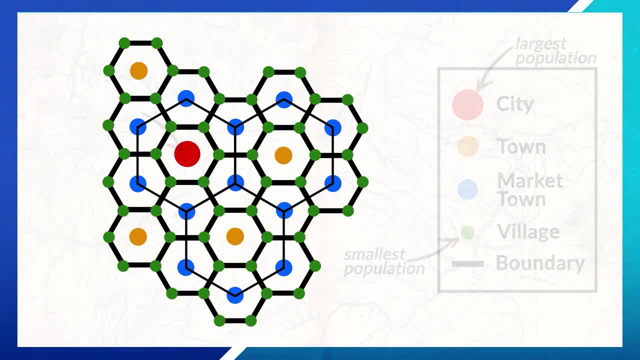 of the region, with smaller settlements located around the larger urban area. The urban area creates a region acting as the economic and cultural hub of the area, as seen here. when looking at Cristal or Central Place Theory, We can also see functional regions such as the. 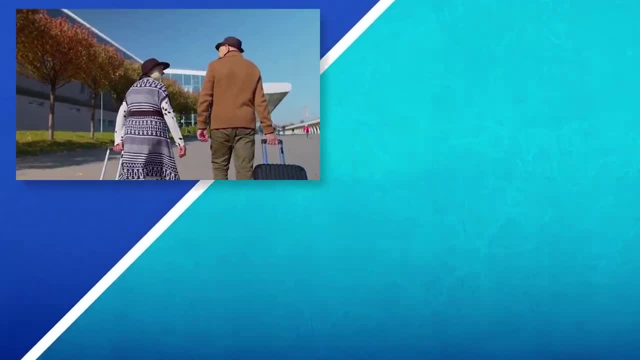 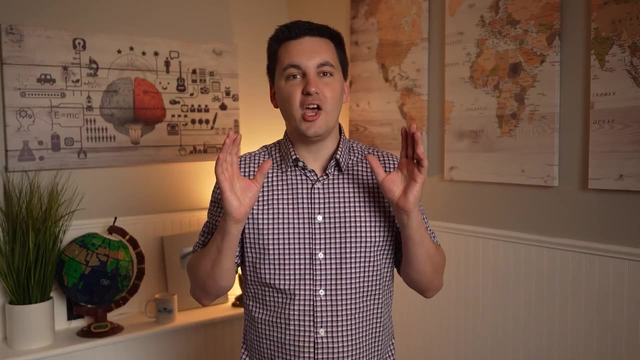 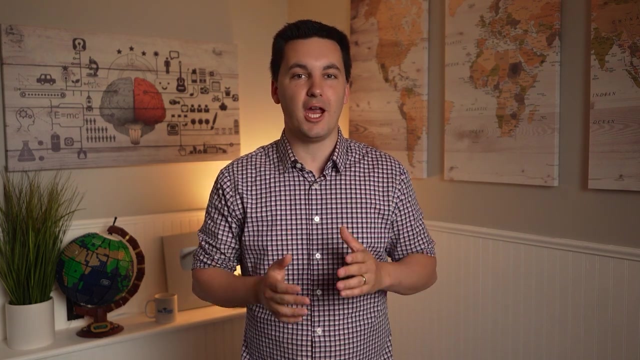 New York City region created by different transportation networks such as airports, train stations, ports or public transportation stations such as subways or bus stops. All of these help facilitate the movement of people and goods between different places and act as a node for the geographic area. 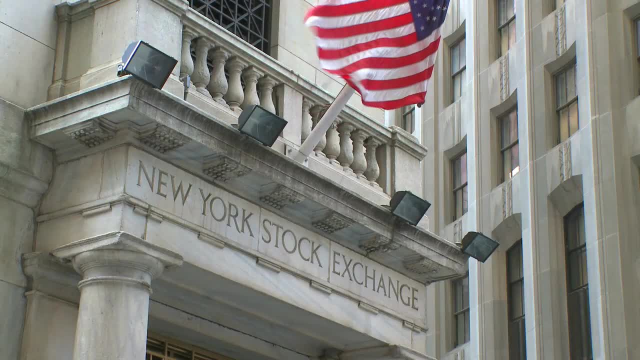 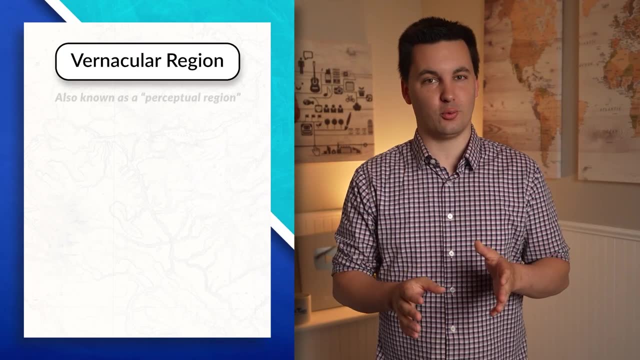 they are located in, Or we could look at financial centers such as Wall Street in New York that serve as a financial hub for investment with the stock exchange. Lastly, we have a vernacular region, also known as a percentile region, which is a percentile region, which is a percentile region. 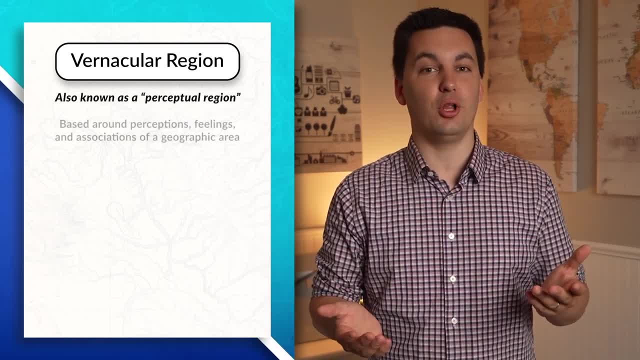 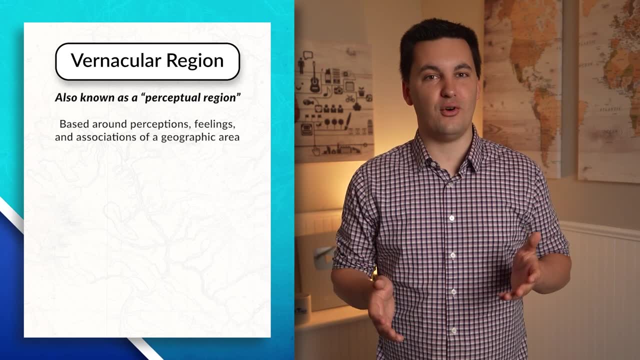 which is a percentile region. This region exists in the minds of the people and is based around their perceptions, feelings and associations of a geographic area. These regions are hard to define since there is no set boundary. For example, what states are part of the American South? 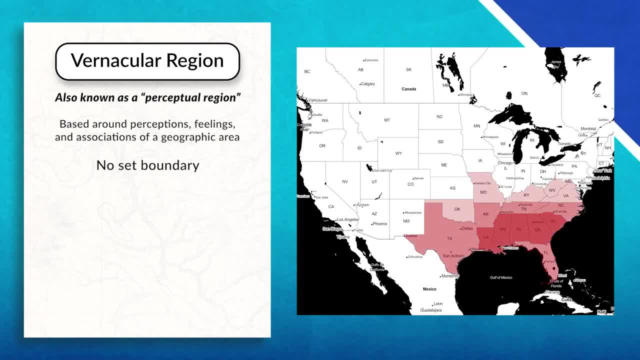 Generally speaking, people think of the South in the United States as having a common cultural identity, shared traditions and also shared history, But the states that are included in the South vary depending on who you talk to. Now, whenever we're talking about regions, 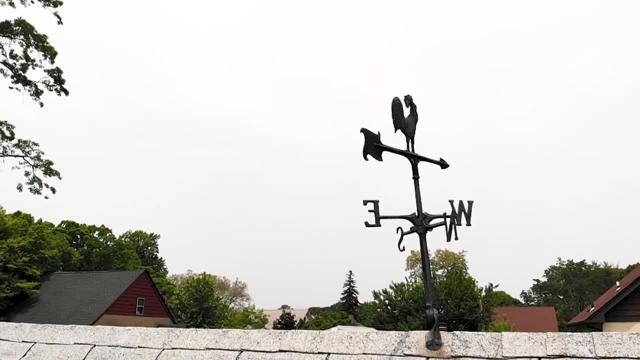 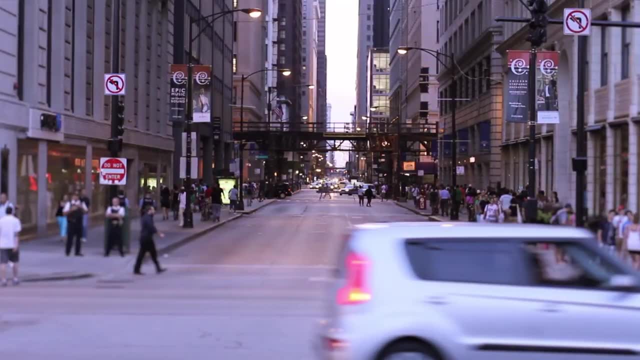 one general rule of thumb that you can use is: whenever cardinal directions are used for a region, the region is most likely perceptual. So we can see that, depending on the geographic area, human activities flow or the topic of discussions, regions can vary, But understanding.